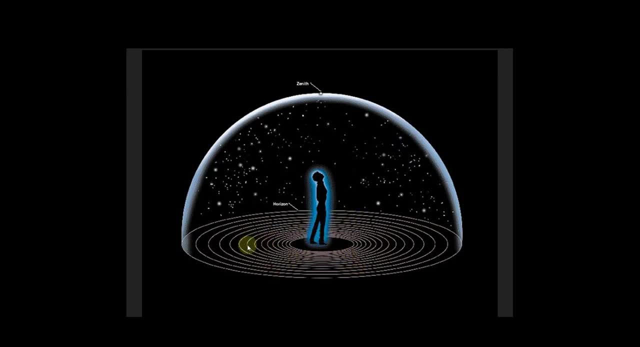 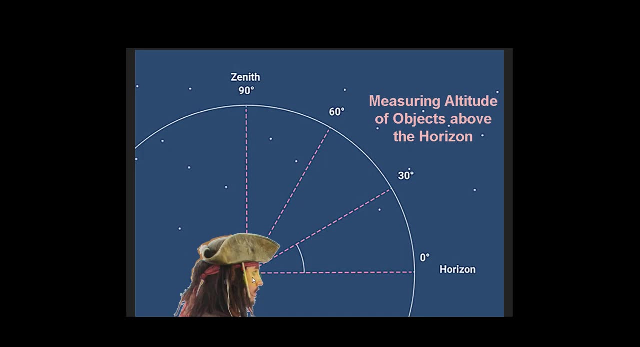 equally far away in all directions. so it's an illusion, but it sure looks real to the observers. When the observer looks at the horizon, he sees the horizon is zero degrees, and so this constitutes the zero degrees at the horizon. You don't always see the zero. 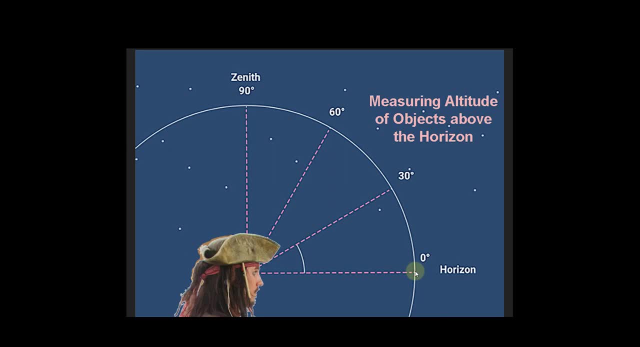 degrees, because most of the time there's a building or trees or something in front of the observer. Now, this is about 30 degrees above the horizon. This is called altitude of the objects above the horizon. This would be a 60 degree altitude. 90 degree altitude is at the zenith. 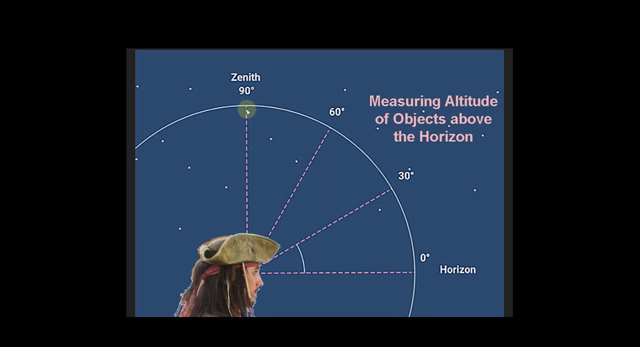 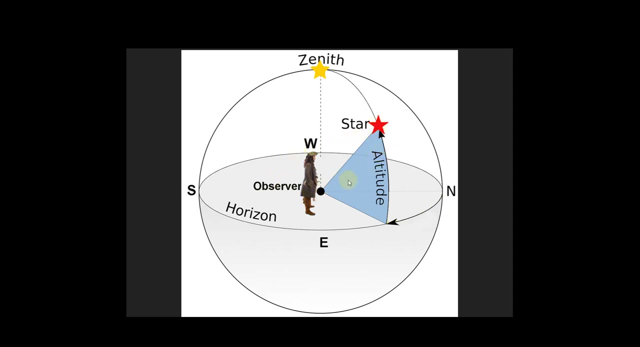 That's the highest point in the sky, and so the observer sees zenith at an altitude of 90 degrees. Now this observer is looking at this red star first, and he notices the red star is about 45 degrees above the horizon. He sees another star, yellow star, at the zenith. 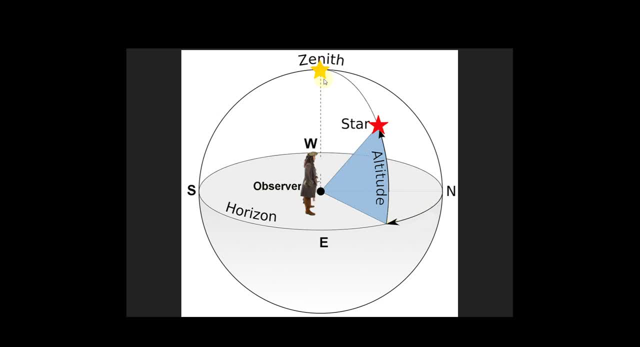 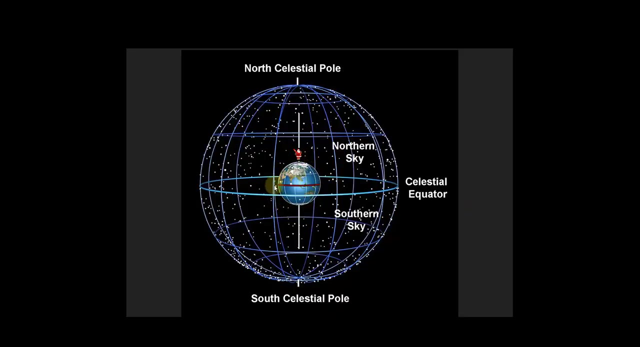 This yellow star is 90 degrees above the horizon, so the altitude of the yellow star is 90 degrees above the horizon and the red is 45 degrees altitude. This is Santa Claus at the north pole of the earth, inside of the celestial sphere. 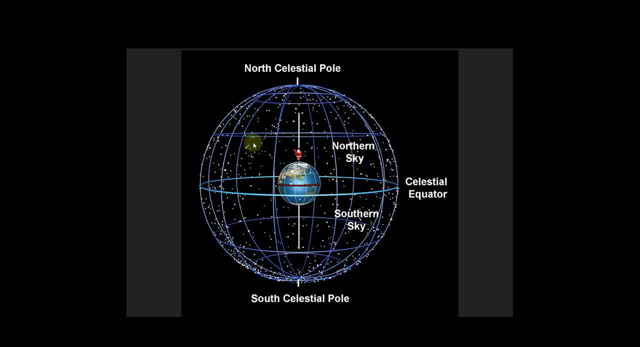 So the celestial sphere surrounds the earth and this is Santa at the north pole of the earth. When Santa looks around, he sees that the celestial equator is actually around his horizon. so that constitutes Santa's horizon, and since the stars are going round and round his horizon, 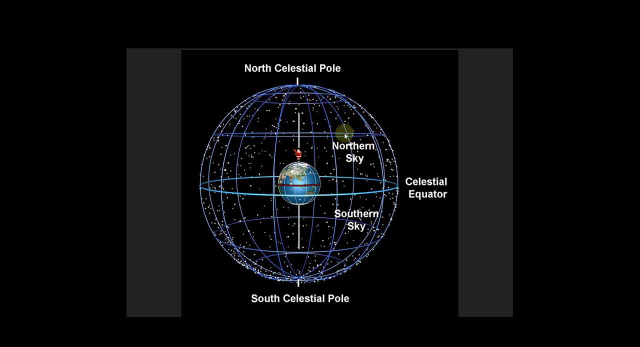 like this, and even if we look a little bit more closely around Santa's horizon, none of the stars at the north pole ever sit-they just go parallel with Santa's horizon. Now Santa moves to the equator of the earth. At this point Santa sees: 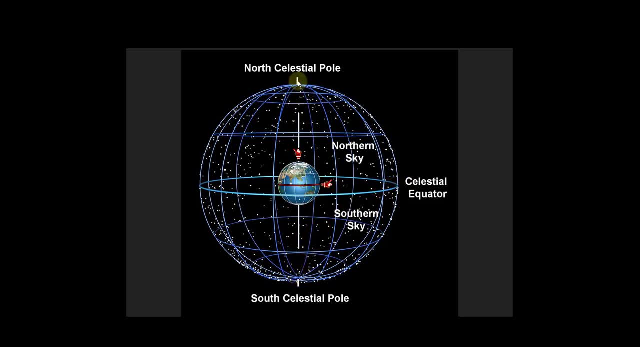 celestial equator at his zenith and he sees the South Selestial Pole and North celestial pole if he just turns around north celestial pole and south celestial pole only from the equator of the earth. if you go on top of a mountain As the earth rotates, Santa will be able to see the other half of the sky as well. 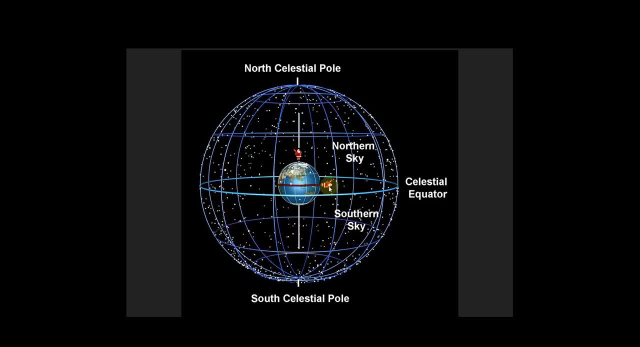 So Santa at the equator will have the chance to see the entire sky. The only observer that can see the entire sky is at the equator of the earth. This is me in San Diego, 32 and a half degrees north. So Santa is at 90 degrees north latitude. This Santa is at zero degrees latitude. I am at 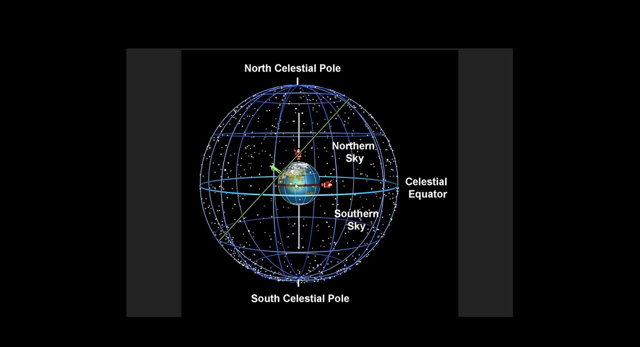 32 and a half degrees latitude. My horizon looks something like this: So how many degrees above my horizon is north celestial pole? Well, since I live in San Diego, 32 and a half degrees north, we can say that the north celestial pole is about 32 and a half degrees. 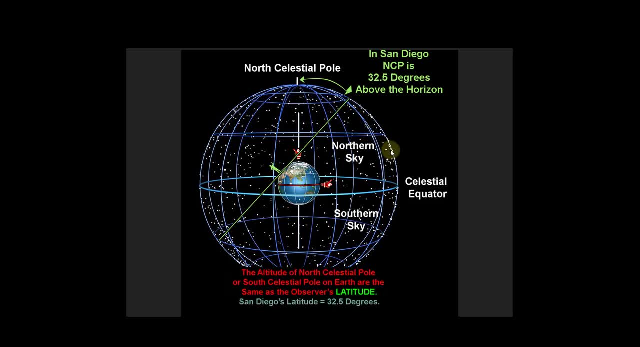 above the horizon. So we can say the altitude of north celestial pole or south celestial poles on earth are the same as the observer's latitude. San Diego latitude is 32 and a half degrees. Therefore, in San Diego north celestial pole is 32 and a half degrees above the horizon. Now we also see. 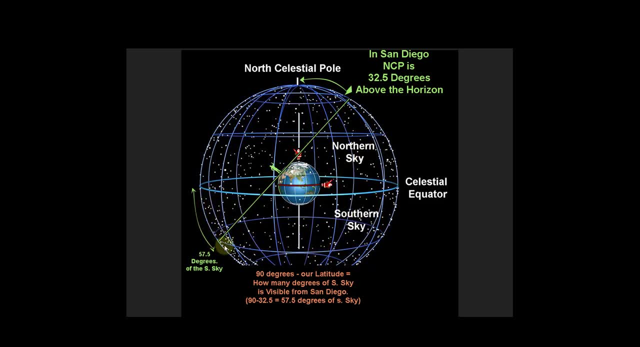 some of the southern sky. This is the southern sky. We see some of it. How much of it do we see? Well, we can subtract our latitude from 90 degrees and then we can find out how many degrees of southern sky is visible from San Diego. So, in San Diego, 90 minus 32 and a half gives us 57 and a half degrees. 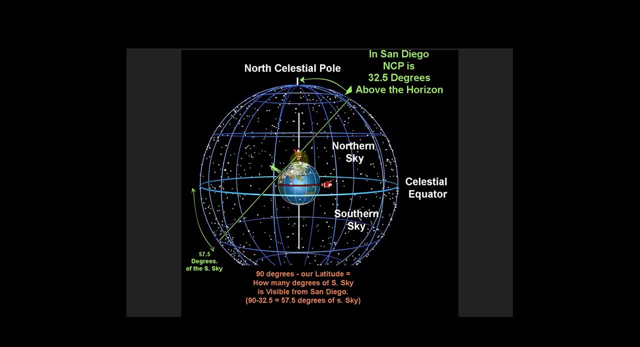 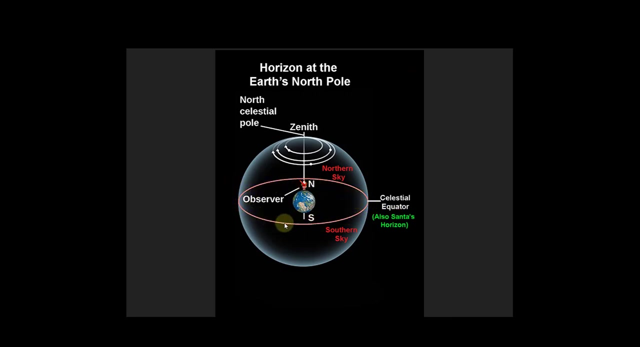 of the southern sky. From Santa's location he sees 90 minus 90 zero degrees of the southern sky. From this location at the equator, Santa sees 90 minus zero. That means 90 degrees of the southern sky. So all of the southern sky is visible to Santa at the equator. This is another view of Santa.